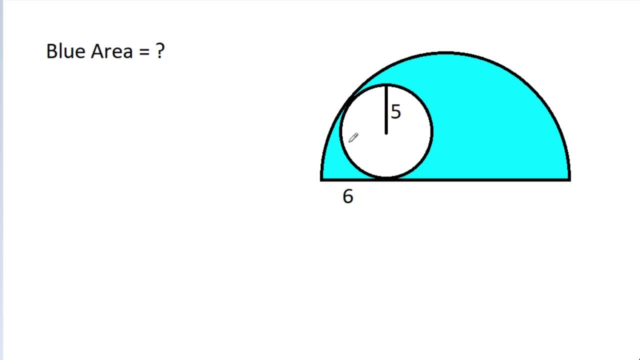 In this video we have given a circle inside a semicircle touching at these two points, and radius of circle is 5 and this distance is 6.. Then we have to find this blue area. So if two circles are touching each other at point Q, then they will have common tangent at point Q. 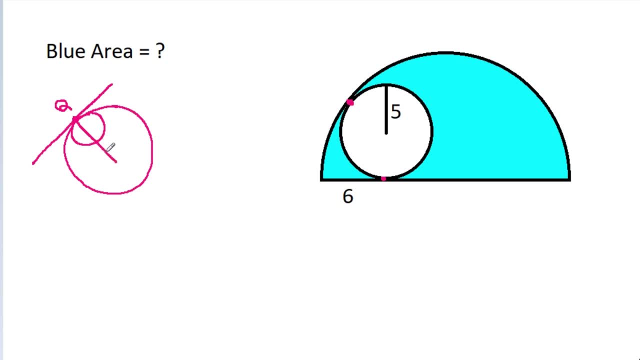 And if we draw a perpendicular at point Q, then it will pass through center of both the circles. suppose O and P, And suppose center of circle is P and center of semicircle is O, And suppose this point is Q, then QP, it will pass through O. 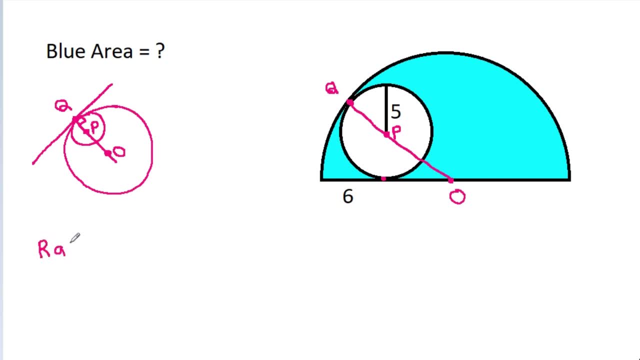 And suppose radius Of circle is small r, It is 5.. And radius of semicircle, Suppose it is capital R, Then QP it will be equal to small r, That will be 5. QP will be 5.. 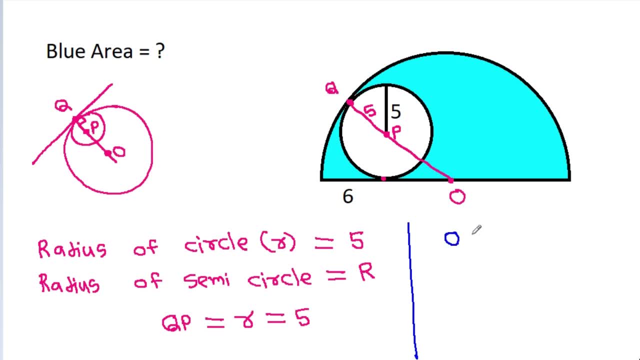 And also OQ will be capital R And OQ is OP plus PQ. That is capital R. So OP plus PQ is 5.. It is capital R. So OP will be equal to capital R minus 5.. OP is R minus 5.. 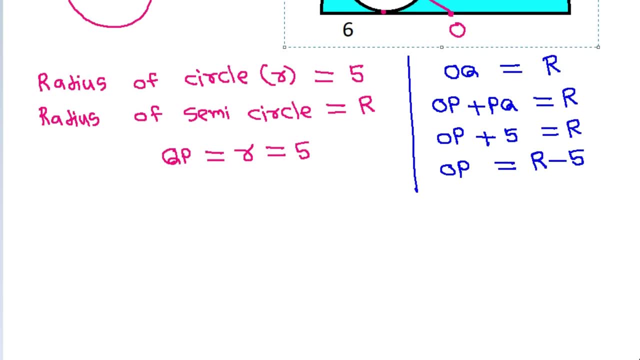 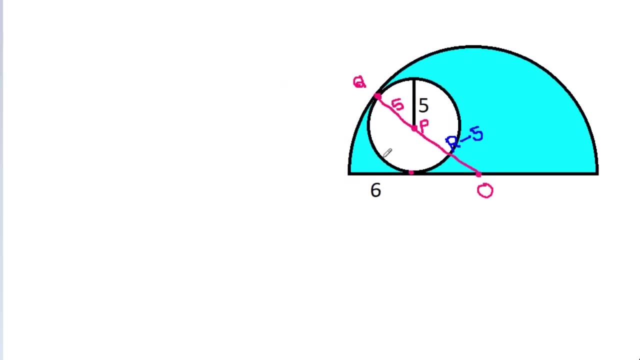 And Now suppose this point is A and this point is B, And if we join PB, then PB it will be small r, That is 5. PB is 5. And OA will be equal to capital R And OA is OB plus BA. 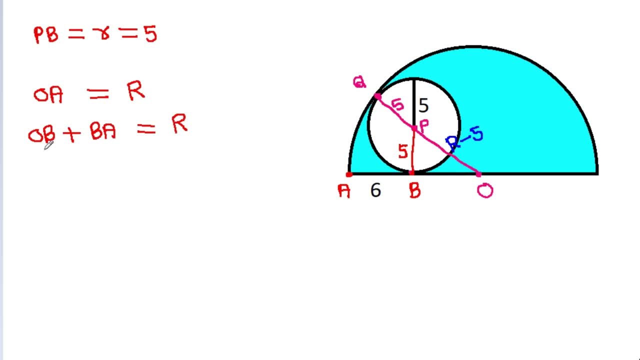 That is capital R, And it is OB plus BA is 6.. That is capital R. So OB will be equal to capital R minus 6.. OB is R minus 6. And in any circle tangent and radius are perpendicular to each other. 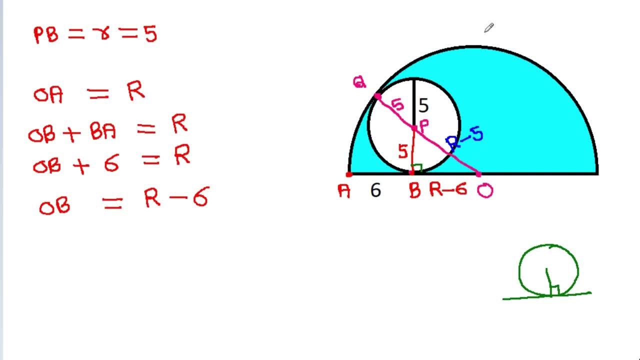 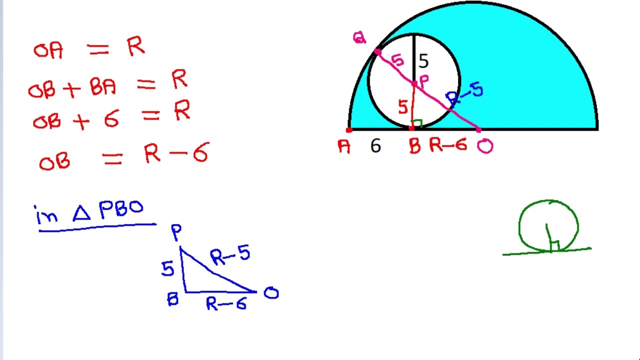 So this angle will be 90 degree. And now inter angle PBO. It is PBO, PB is 5.. BO is R minus 6. And PO is R minus 5. And this angle is 90 degree. 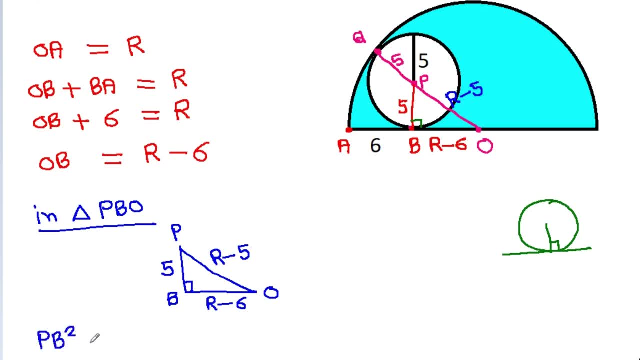 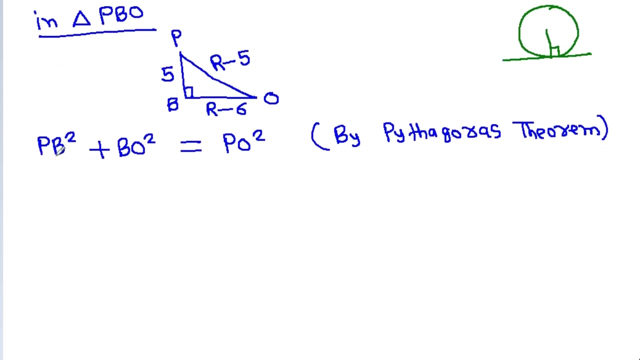 So PBSQ, PBSQ plus BOQ, It will be equal to POSQ by Pythagoras theorem, And PB is 5. Sq Plus BO is R minus 6. Sq- It is equal to. PO is R minus 5.. 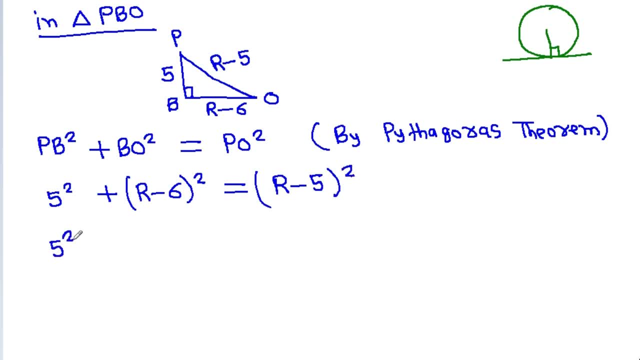 Sq And it is 5. Sq Plus, And this will be equal to R Sq Plus 6. Sq Minus 2 times R times 6. It is equal to R minus 5. Sq- It will be R. 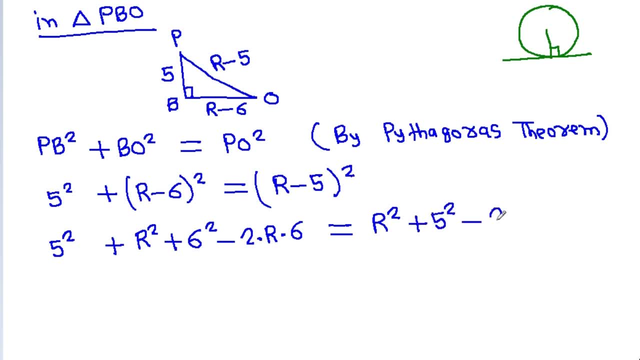 Sq Plus 5. Sq Minus 2 times R times 5. And R Sq Will get cancelled. 5. Sq Will get cancelled And 6. Sq Is 36. Minus 12 R. 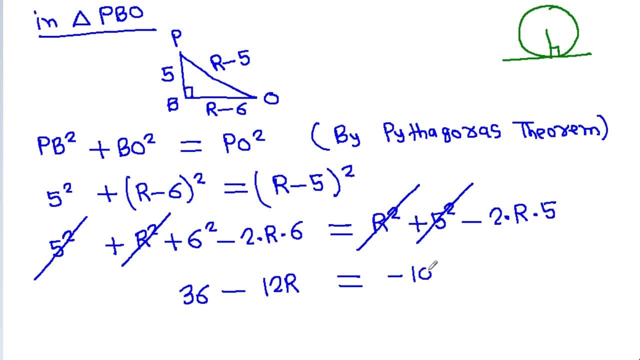 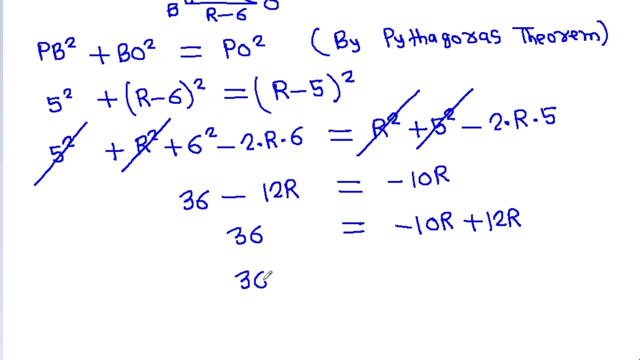 It is equal to Minus 10 R And 36.. Will be equal to Minus 10 R, Plus 12 R And 36.. Is equal to 2 R, So R will be equal to. 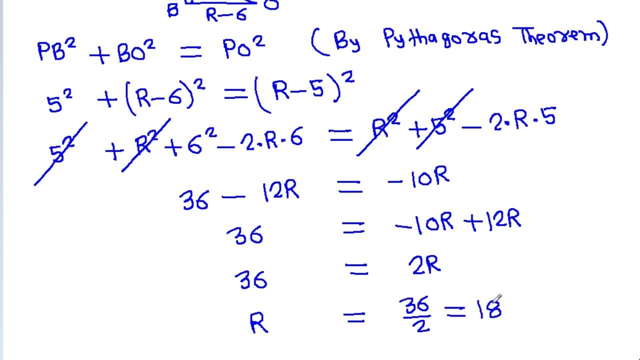 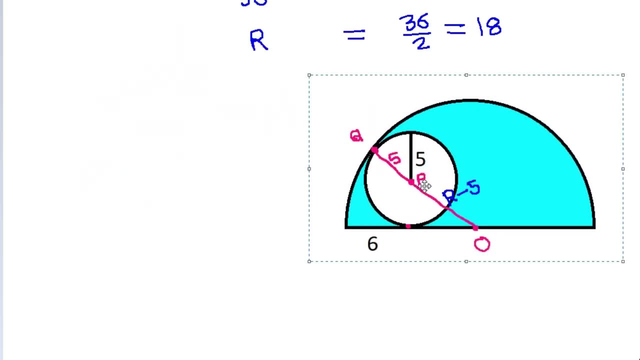 36 by 2. That is 18.. And Now Blue area. It will be equal to Area Of Semi circle Minus Area Of Circle, And Area Of Semi circle It will be 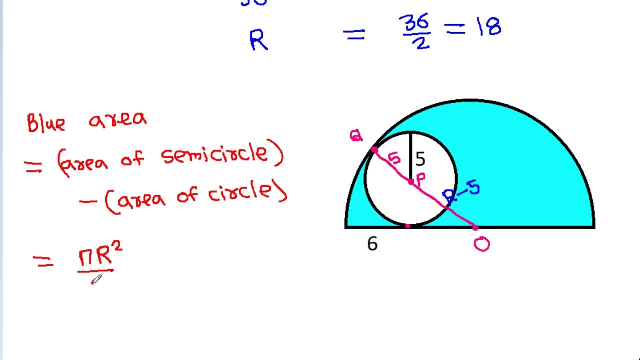 Pi Times R? Sq By 2. Minus Area Of Circle It will be Pi Times R? Sq And It is Pi And R Is 18. Sq By 2.. 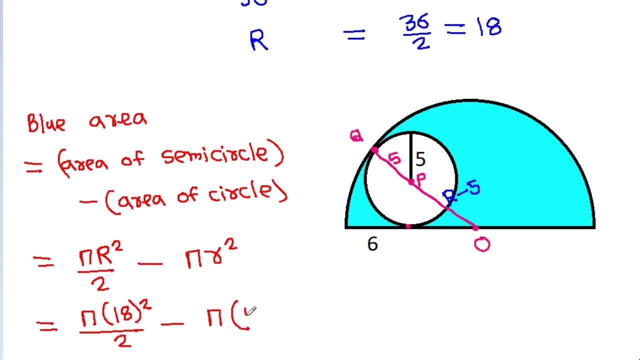 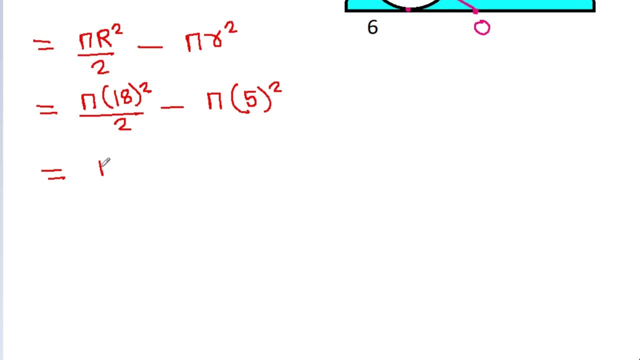 Minus Pi Times. Smon R Is 5. Sq And It is Pi Times 324.. By 2. Minus Pi Times 25. And 2. Times.